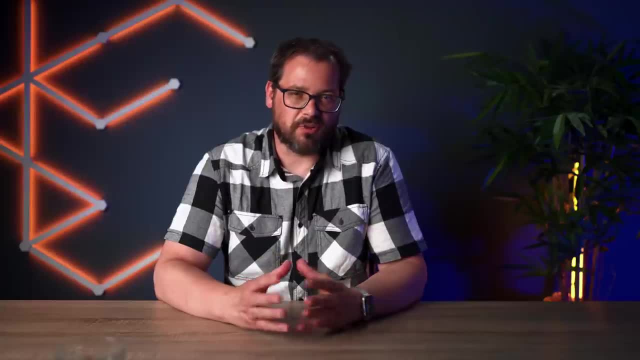 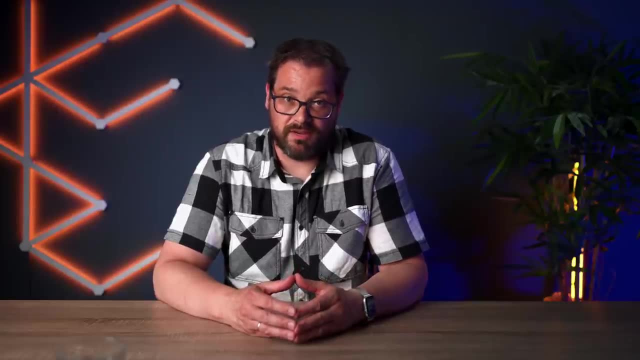 If you don't, you're going to run into incompatibility issues. The software might crash in the cloud but work perfectly on your machine, and that makes testing things and fixing those issues a real pain. So today I'm going to show you how to go all in on Docker and avoid all of. 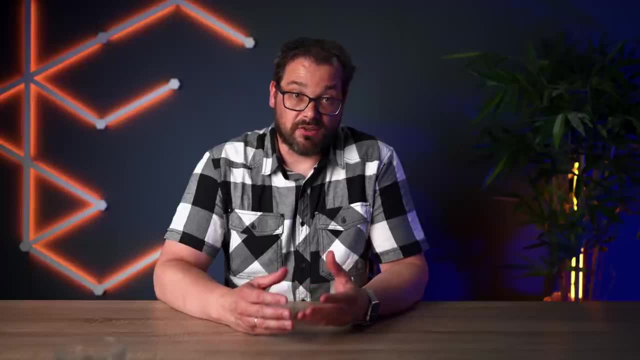 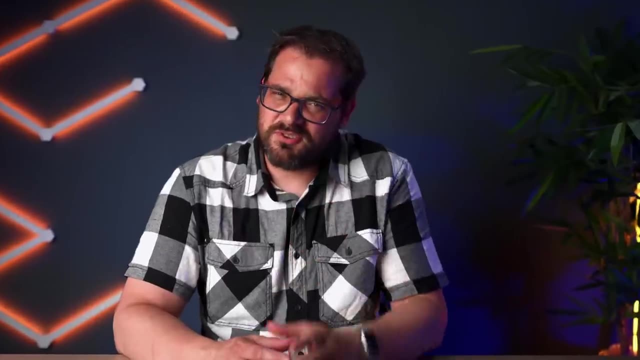 those problems, And I'll use a simple API server in Python as an example. The code for this episode is on GitHub, including all the settings. It's ready to go, so you have no excuse to not do this. Well, maybe one: You might not have thought through all the necessary steps to design your software. 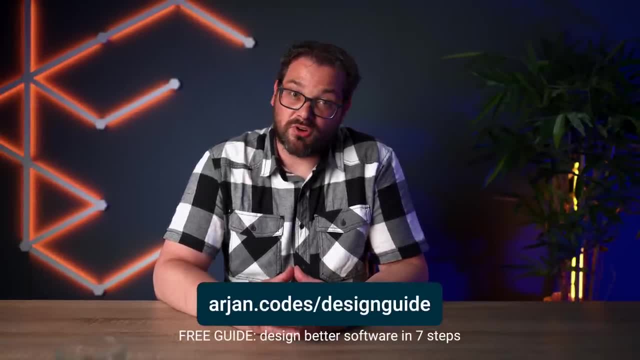 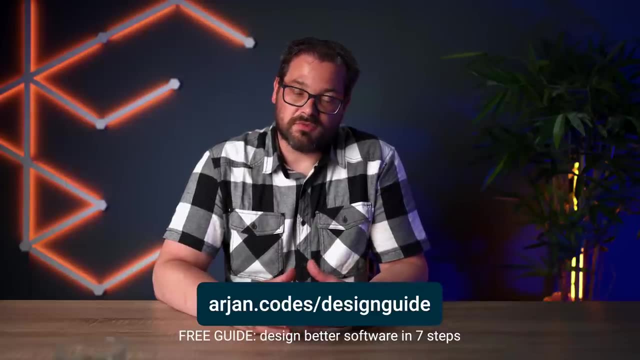 and for that I have a free guide for you. You can get it at arjoncodes slash design guide. It contains the seven steps I take whenever I design a new piece of software. I think it'll help you avoid some of the mistakes I made in the past. 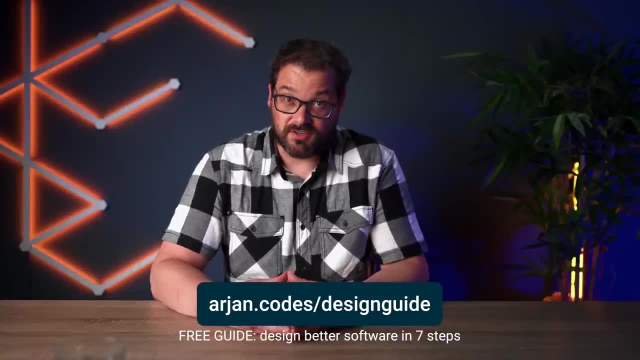 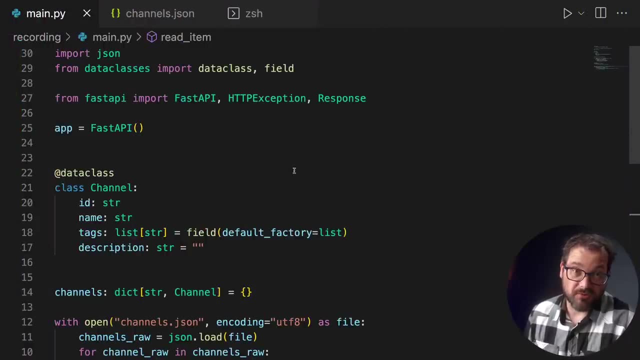 and put you on the right track. So arjoncodes slash design guide. The link is also in the description. This is the code example that we're going to use today. It's a simple API that retrieves YouTube channel information. I'm not even accessing the YouTube API, I'm just 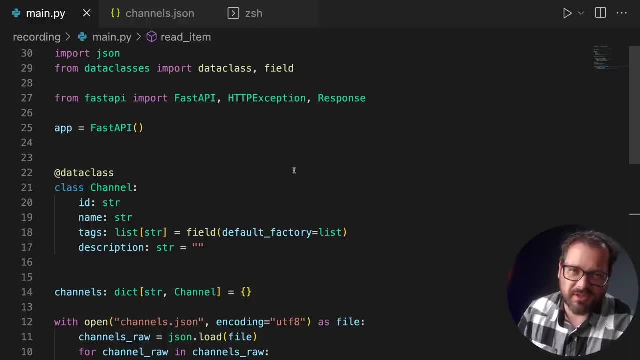 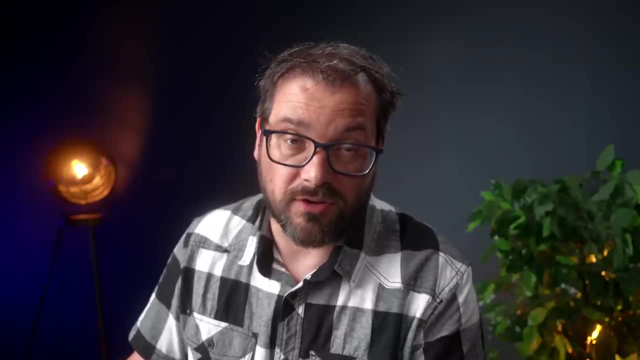 reading that stuff from a JSON file that I just put in here to keep things simple, And later on I also want to show you how to deal with data and syncing data between local folders and your Docker container, which is actually really simple, But what I have here is pretty basic built. 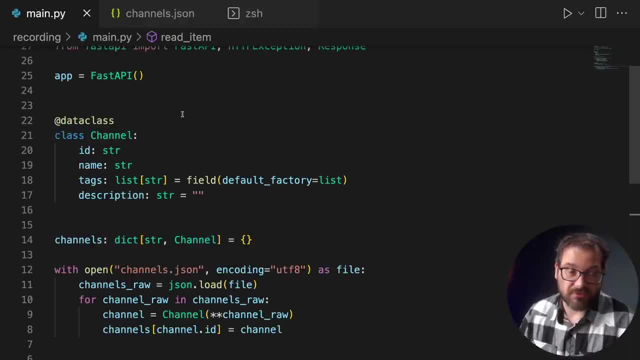 on fast API. I'm defining a class called channel, which represents a YouTube channel that has some information like the ID, the name, some tags and description. What this is exactly doesn't really matter- And then I read the channel information from a JSON file. Normally you would use a. 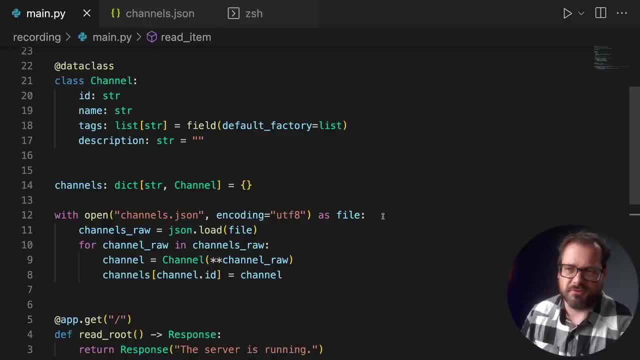 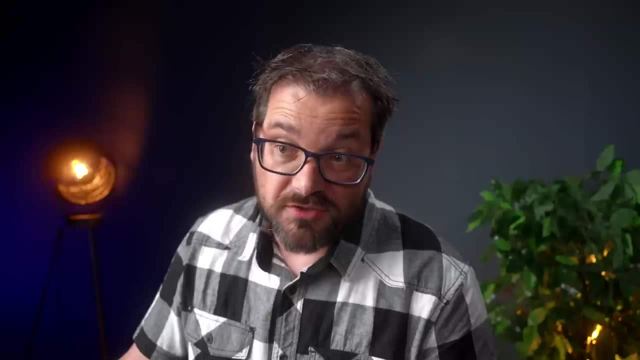 database, but I want to keep it pretty simple in this example, so I just use a file, And this file just contains information about a couple of different channels. There's CodeStacker, Jack Harrington and myself. These two channels, by the way, are really nice. You should check them out if you haven't done so. 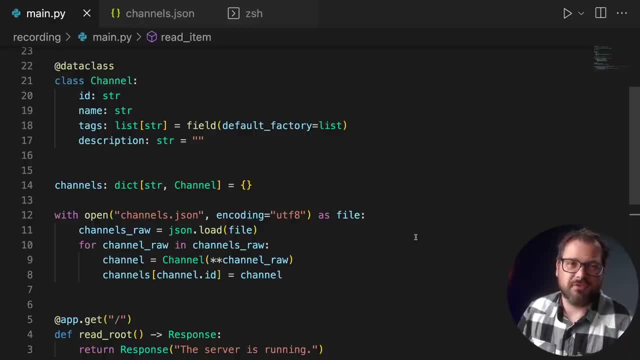 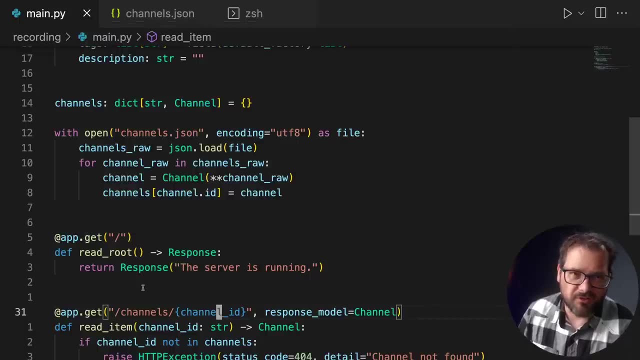 So there's basically only two types of requests you can do in this particular very simple server. One is a simple GET request at the root, which is like a health check of the server, So it just returns the response that the server is running, And then there is another GET request. 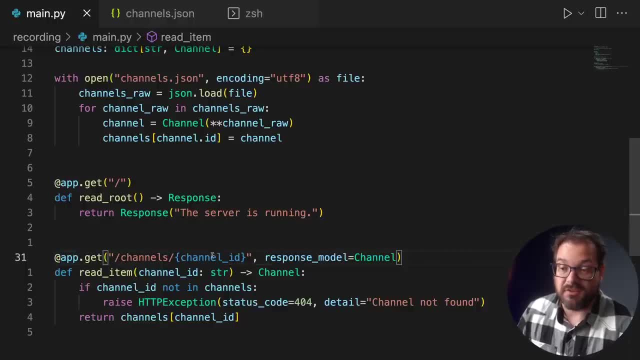 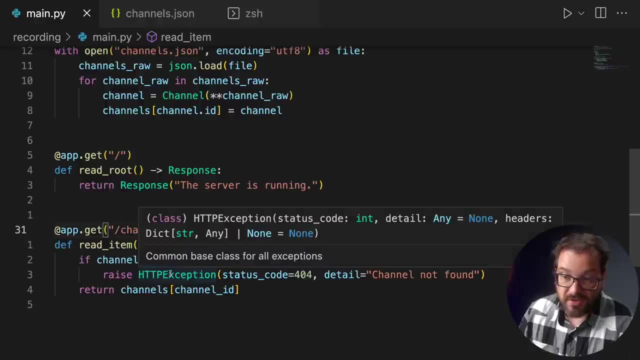 that allows you to retrieve a channel based on the ID that you provide, And the only thing that this does is it checks. if the channel ID is not there, Then it raises an exception. That's a status code 404.. Not found Error. 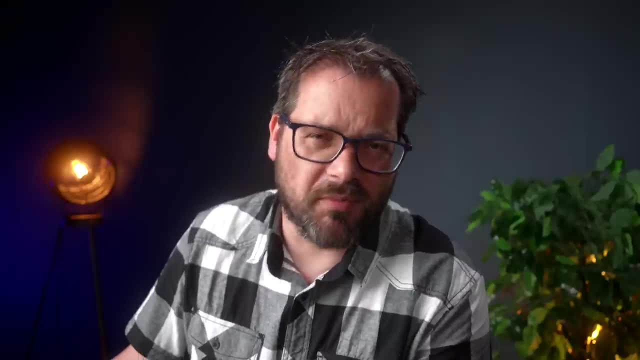 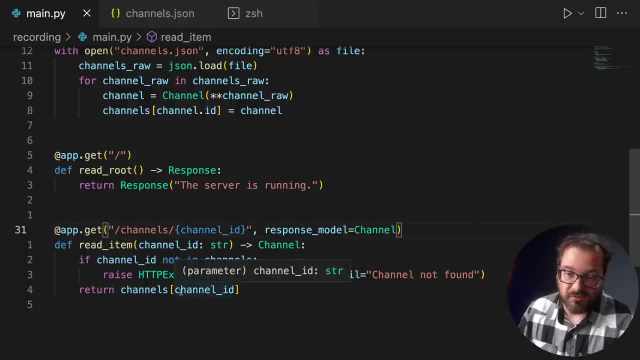 And it gives some detailed information. Well, not that many details. Channel not found, And if it is there, then it's simply going to return the content of the channel at that particular ID. Also again here, this is really simplified. You wouldn't do it this way in a production API because you want to. 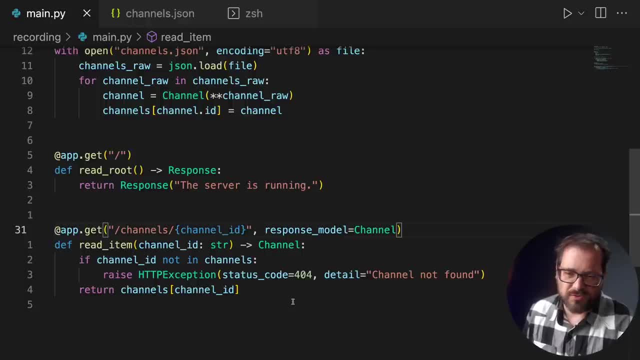 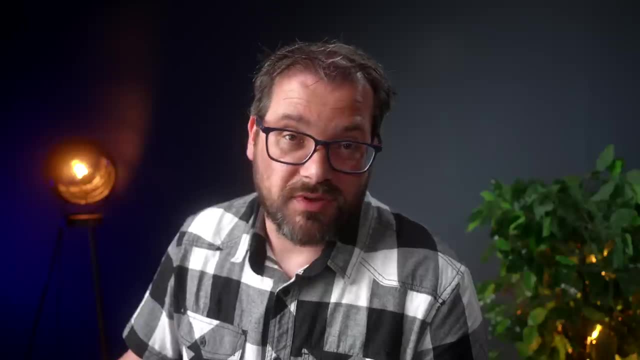 separate those things a bit more. I have a whole section in my online course where I talk about this topic in detail, But here I just want to keep things really simple. So this is how I did it in this particular example. So in principle, that's all you need to set up a channel. 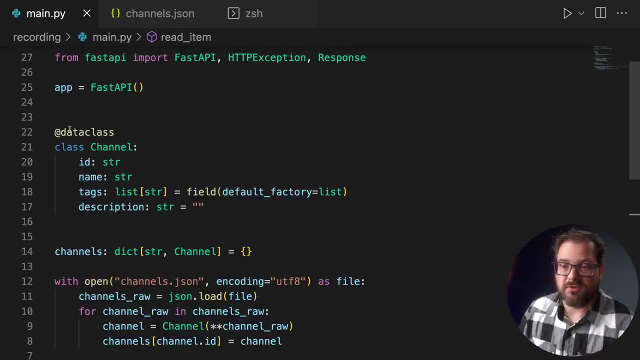 A really simple API. One thing I want to mention is that you see that I'm using a data class here to represent the channel. You can also use Pydentic if you want to. Fast API supports Pydentic And Pydentic is actually compatible with data classes, So that's why we can also use a data. 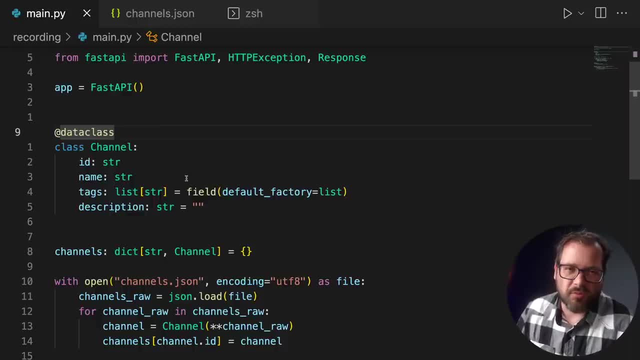 class here, And this example I'm showing you here is actually also very similar to the basic example that Fast API itself shows on their homepage. So how do we run this server? Well, for that we're going to use UVCorn, And UVCorn allows you to run. 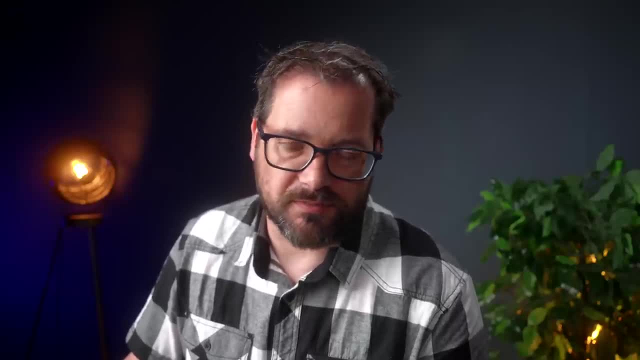 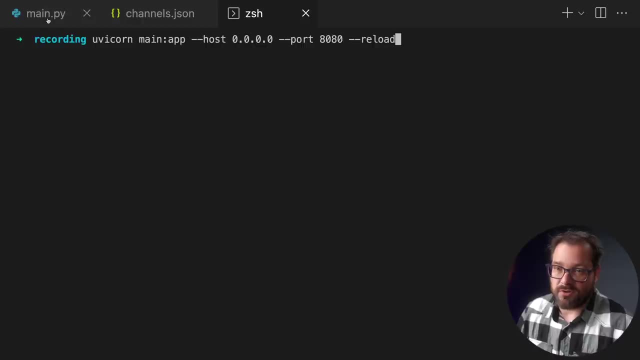 a server like this and expose it to a particular port. Here you see the command that you need to run in order to start the server. So, along the main file, that's the app server, which corresponds to this variable here, And the host is local. That's the local host And the server is accepting. 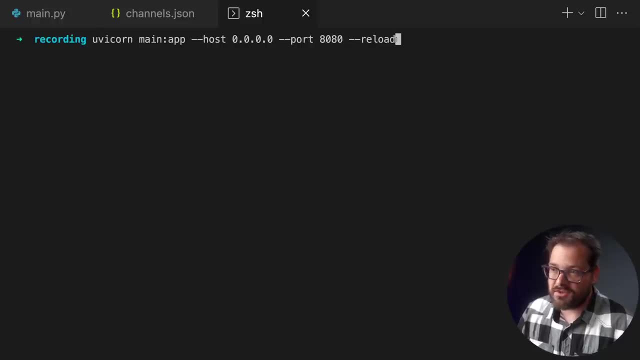 request on port 8080.. And there's also this dash dash reload. That means that if we change things in the file then the server is going to automatically reload so we can see the effect of our change. So when I run this you see we get some status messages here. It started the server and we have. 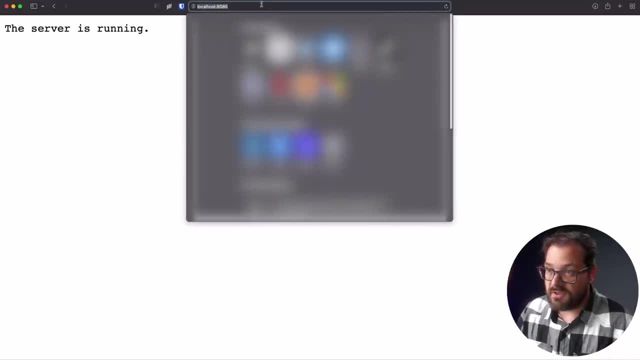 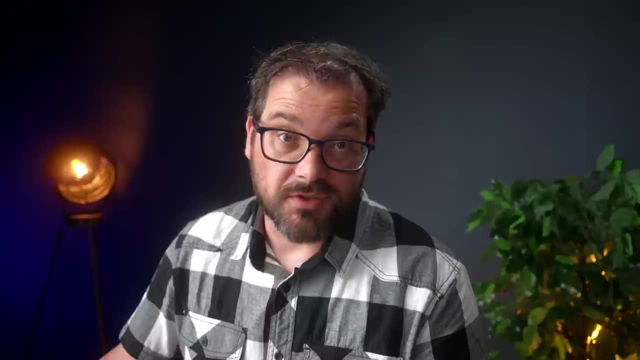 the link here And then when I do the simple get request, you can see it here. That's simply local host at 8080.. We get that the server is running, which is what we expect, And now we can also use the channels endpoint to get YouTube channel information, For example. I could get the information. 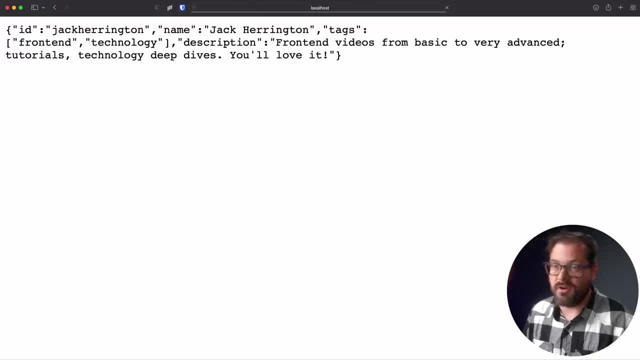 of the channel by Jack Harrington, like so, And then I'm getting JSON data back. If I make a mistake here and I accidentally write it in the wrong way, then I'm going to get the 404 error with the detail that the channel wasn't found And, because of the reload option, if I change things, 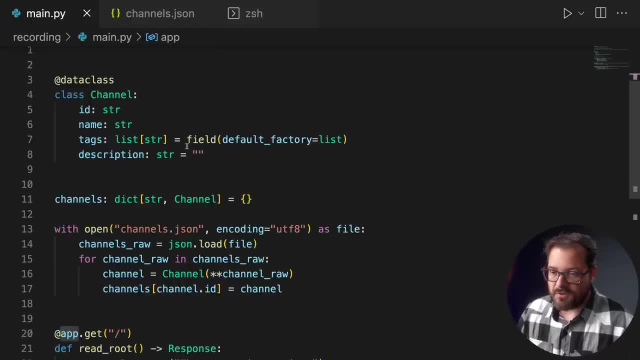 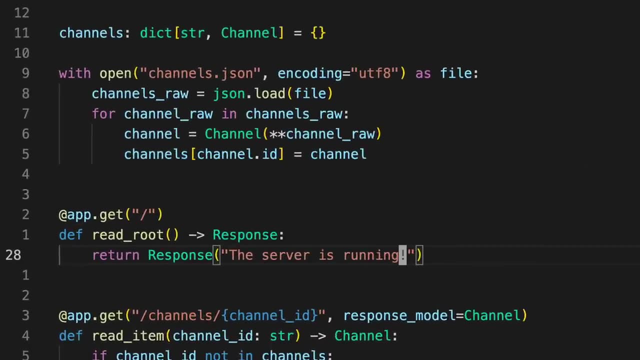 here in the code it's going to automatically reload the server. So, for example, let's say I'm changing this not to the server is running, but the server is running- exclamation mark. So then we get this. I save the file And if we look in the terminal you see that we get here a reload message. 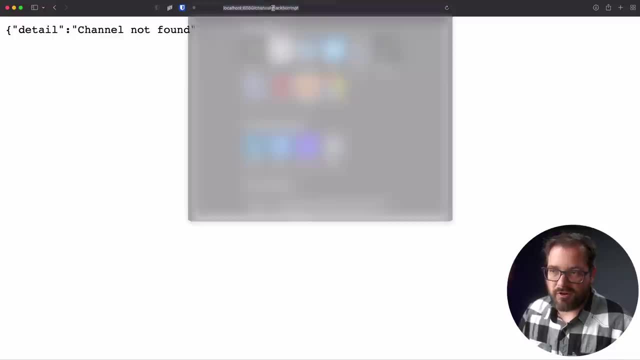 that detected changes in main API and its service. So that's what we're going to do here, And then we're going to go to main API and it's reloading, And now if I load the root folder again, then this is what we get. 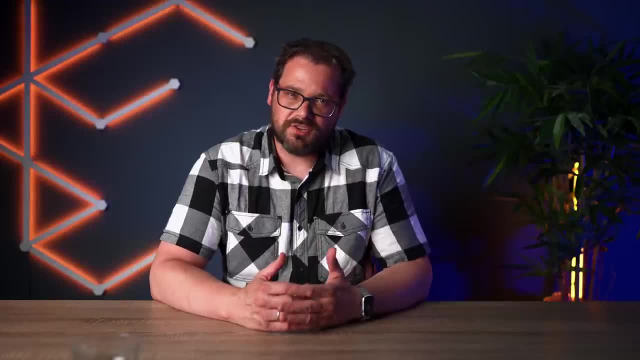 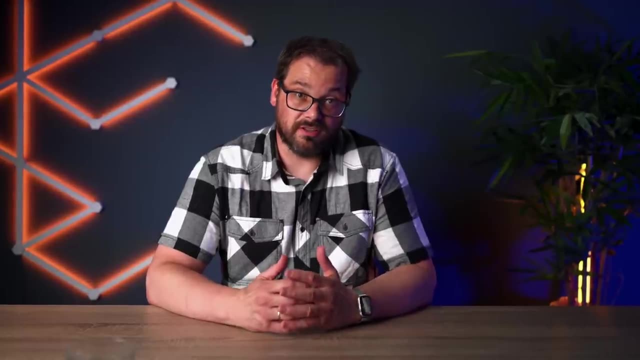 which is the changed code, which is great. Docker has completely changed the game for cloud development. It allows us to run applications in an isolated environment, A container running your preferred Linux distribution. Moreover, you can create an image where you can pre-install software. 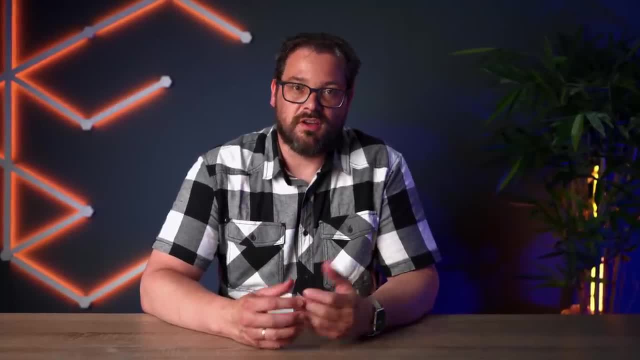 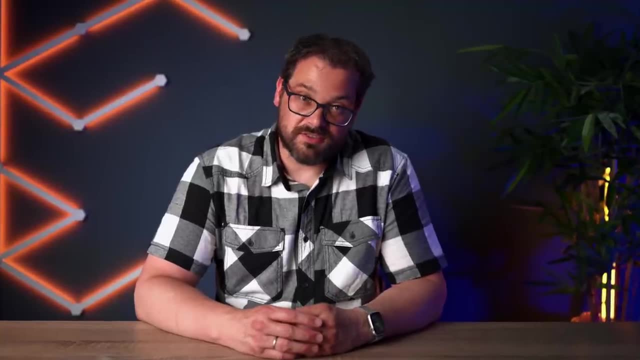 change anything you like, treat it like a virtual machine. You can run these images locally on your machine and they also neatly integrate into the server. So that's what we're going to do here, And that's why this is great with cloud technology, such as Kubernetes. 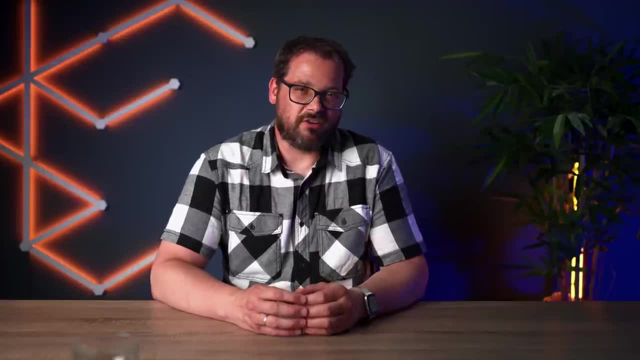 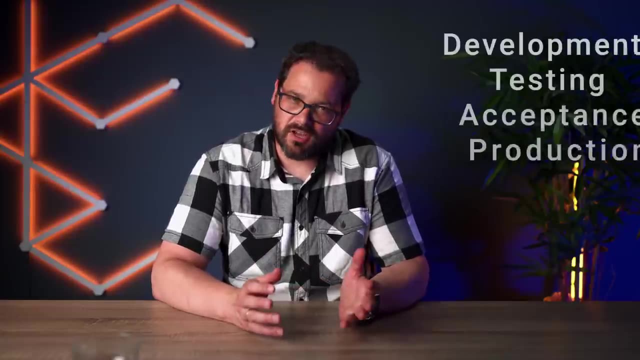 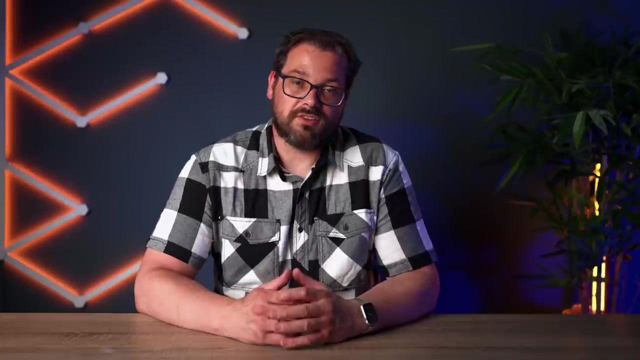 If you're developing a cloud-based app, you're going to have different environments in which the app will run. The classic set or sequence of environments is the DTaP street. but no�there are alternatives to DTaP as well. For example, instead of a sequence, a street, you could create parallel environments For. 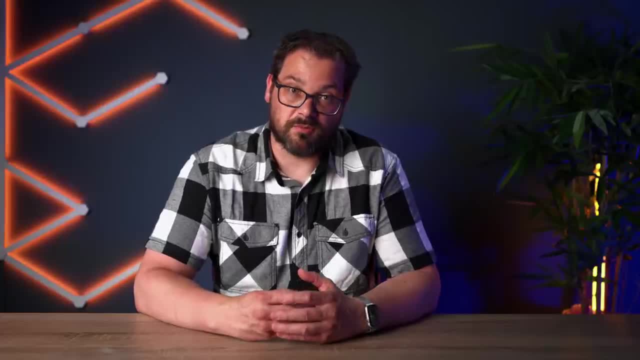 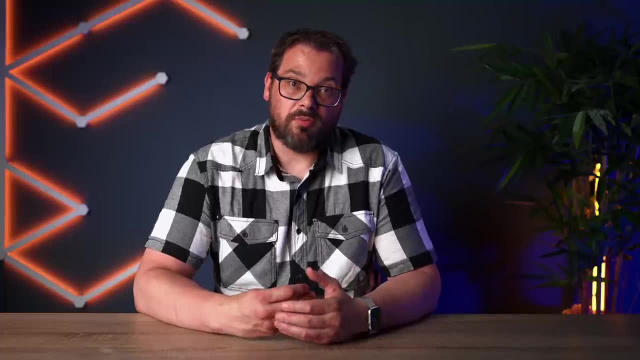 example, have a parallel testing and performance analysis environment. You could do progressive deployments, deployments with feature flags or ring-based deployments that open up a new release to groups of users in sequence. Many possibilities, but I won't talk too much about deployments today. 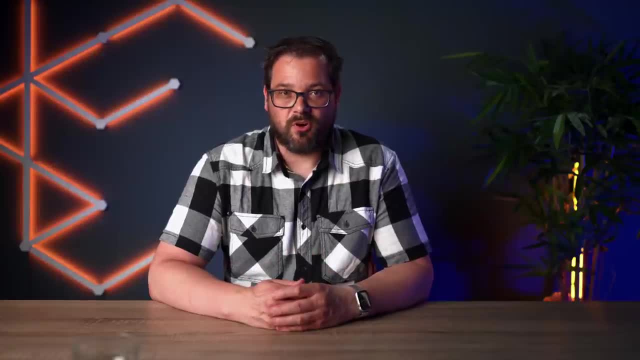 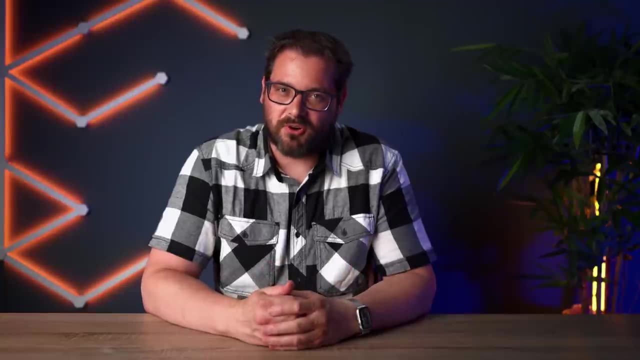 If you'd like me to do a separate video about that, let me know in the comments And when you're there, why don't you hit that like button as well? It really helps me a lot to reach more people. Now back to Docker, Because the same Docker image runs in each of the different environments. you 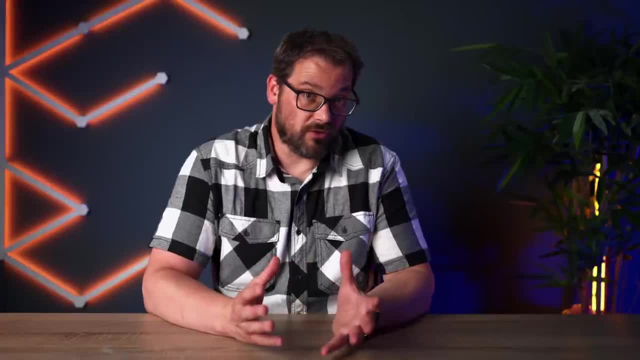 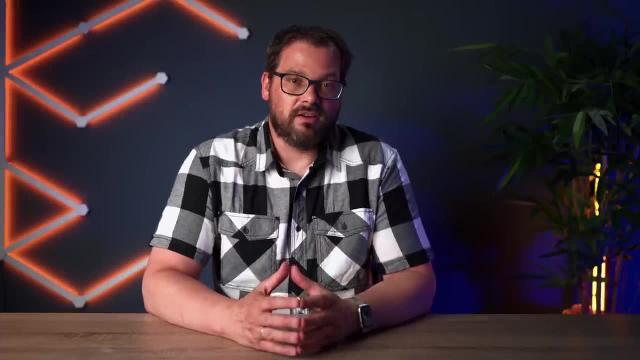 have you reduce the chance that code that runs locally on your machine breaks when you try to run it in another environment. And also having the same environments everywhere simplifies things like testing your code, doing security checks, audits, and it also makes sure that the developers 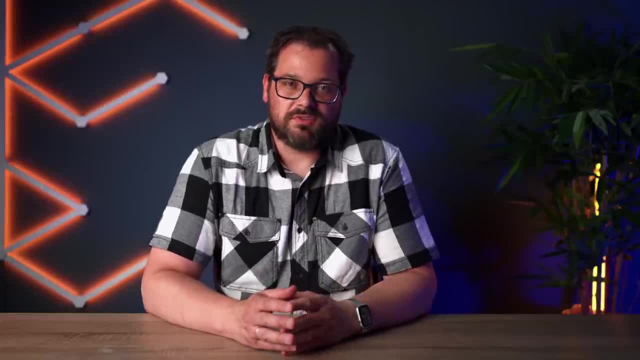 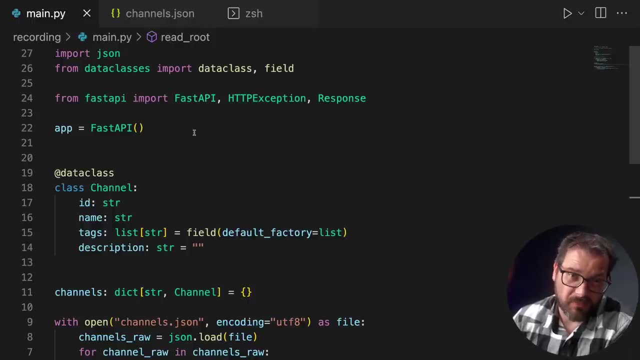 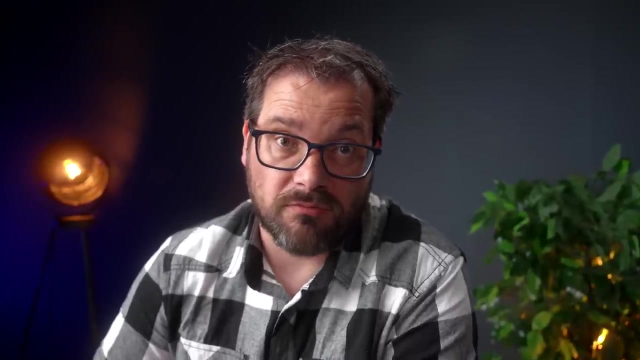 on your team work in the same environment, reducing the potential for errors. The way I'm running this code locally at the moment is not really ideal. I'm running this on a Mac and our server is going to run on Linux, So if I were to deploy this API as is, the server might break for some incompatibility reason between. Mac OS and Linux. I don't know. I haven't tested that And I can't test it because I'm running it on a Mac machine locally and not on a Linux machine. And it's not just the difference in OS that's an issue. 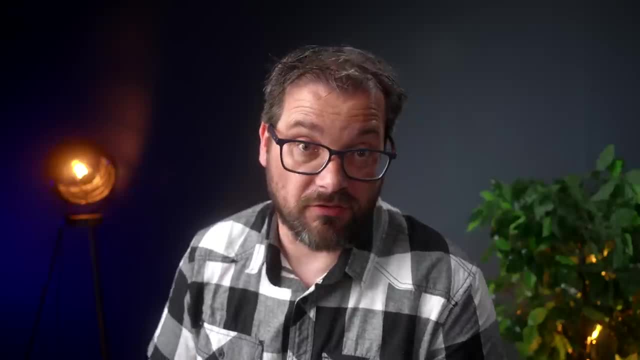 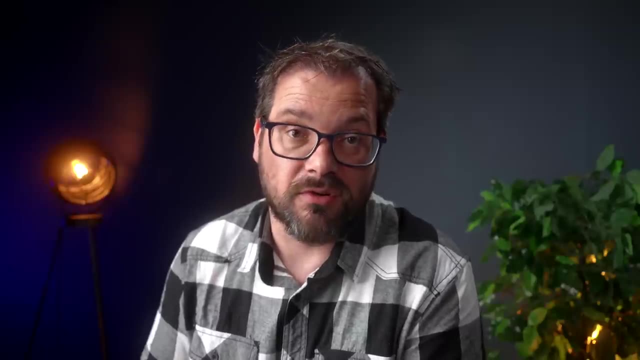 For example, I'm running a particular version of Python on my Mac, I have to verify that the one that's running on my server is going to be the same, And I have to also make sure that the dependencies that are needed in order to run this API locally are the same, And I have to also make sure that the dependencies. 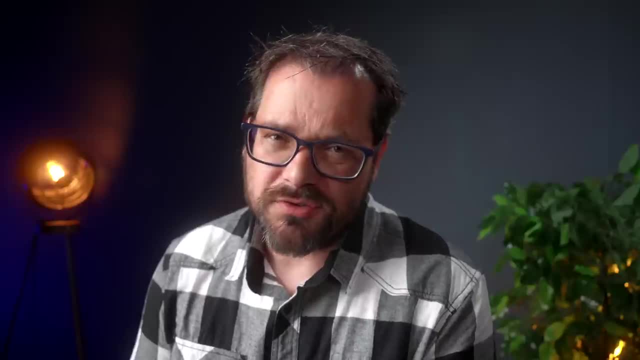 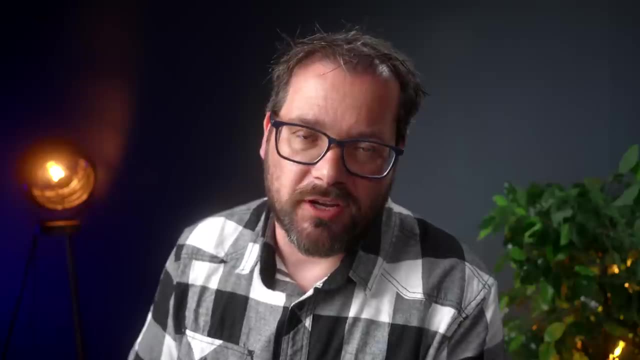 that are needed in order to run this API locally are the same, And I have to also make sure that the dependencies locally are actually installed on my machine. If you're a solo developer working on a project that nobody else is really going to run the code of on their machine, then that might be fine, But as soon 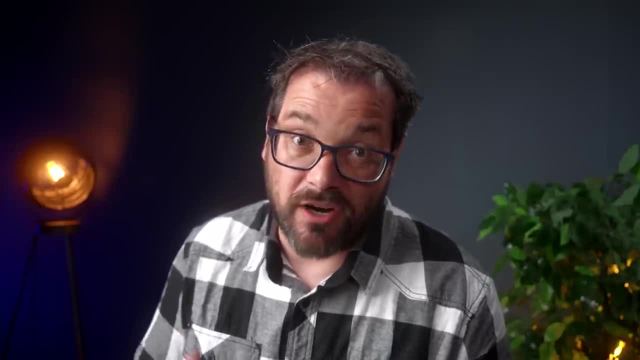 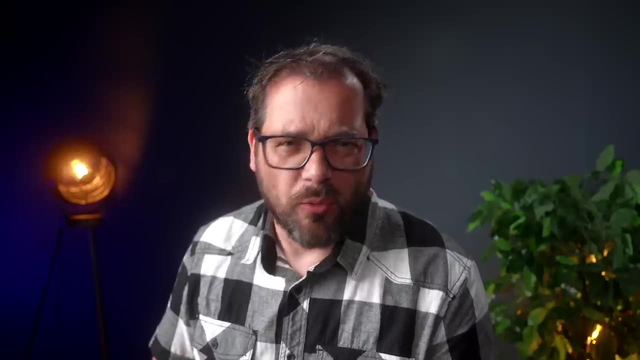 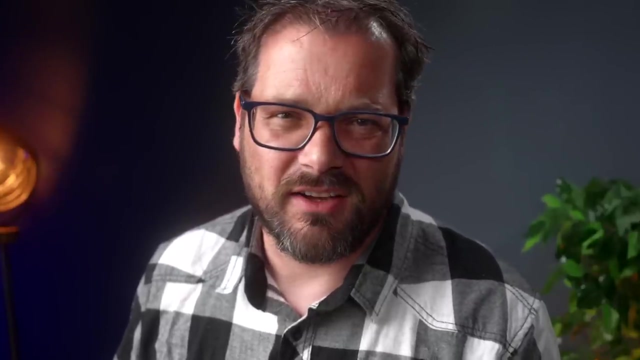 as you're working in a team, it makes a lot of sense to try to make the environments that the different developers in your teams work in are as similar as possible. Basically, anything you can do to homogenize, homogenize, homogenize, homogenize, homogenize: make things the same. 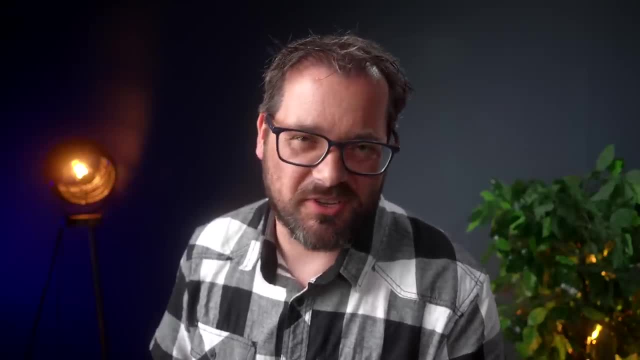 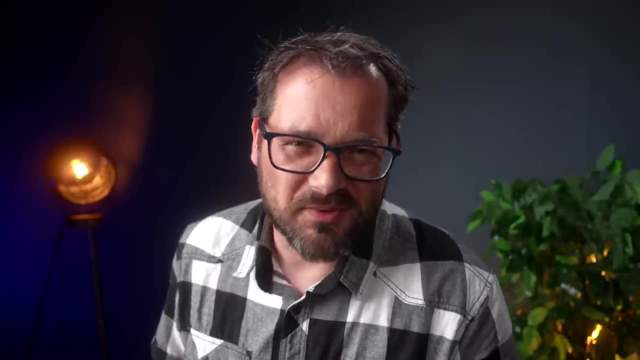 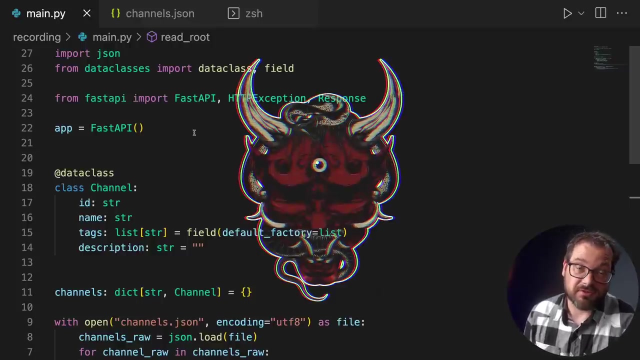 between developers. anything you can do to achieve that is going to make your life a lot easier. I should use less expensive words on this channel. So instead of running this locally, let's try this with Docker. So first, of course, you have to make sure to install Docker, And once you do, you're going to have a Docker daemon. that's 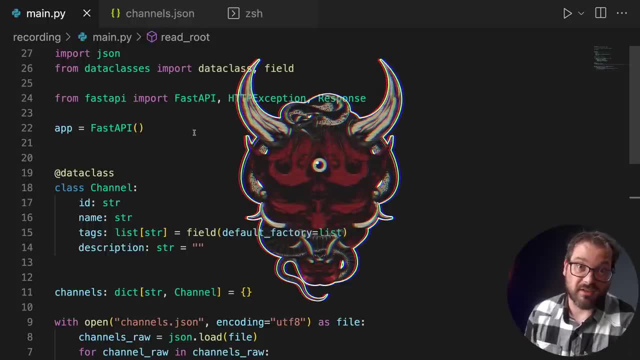 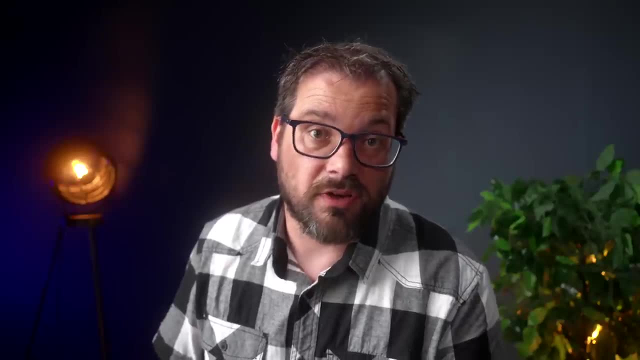 going to be running in the background that's going to take care of running and maintaining your containers. Docker is a really nice tool because it provides a complete virtual environment, a virtual machine on which your code is running, And you can precisely define the kind of environment that you want. So which? 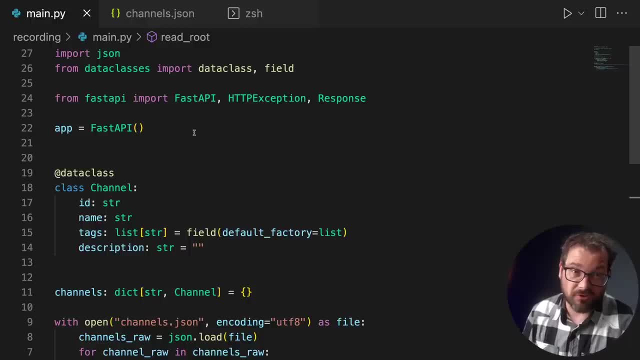 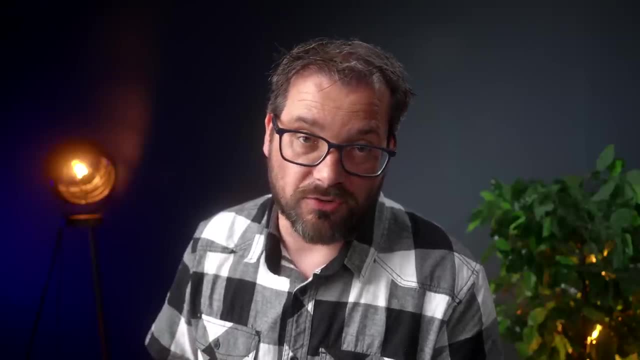 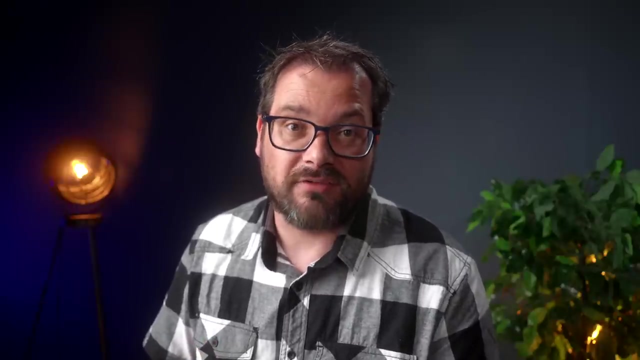 version of Linux. you can supply commands to install things on that virtual machine, And Docker is smart about handling this, So it's going to cache the things that don't change while you're updating the code. And the way that it works is that you create a Docker image according to the settings that you want And then, once you have, 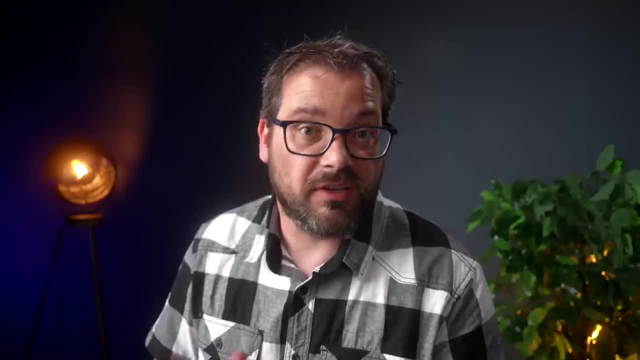 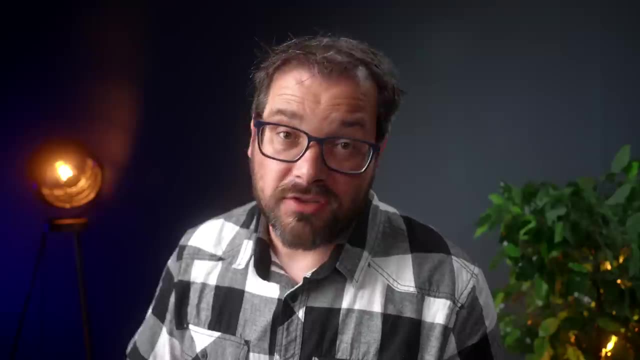 that image. you can run that as a container, And the fun thing is you can locally. you can do that on your server. it doesn't matter. it's the same environment, which is what makes it so powerful. After you've installed Docker, what you need to do is 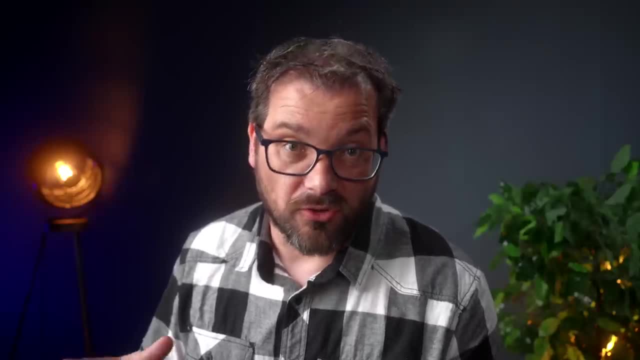 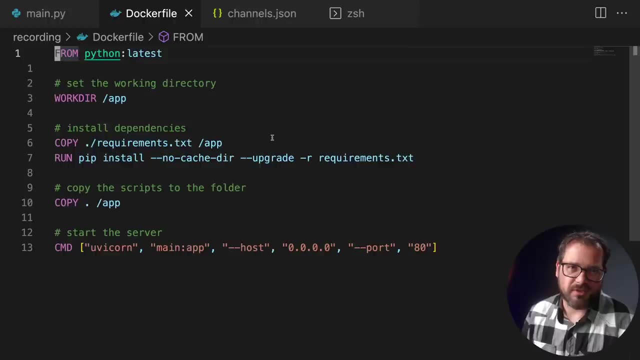 supply a definition, a specification of what you want the Docker image to look like, what are your environment settings basically, And for that you need to define a Docker file. Here you see an example of the Docker file that I'm using for this particular project. The first line defines the image that this image is going to be built on, And that's 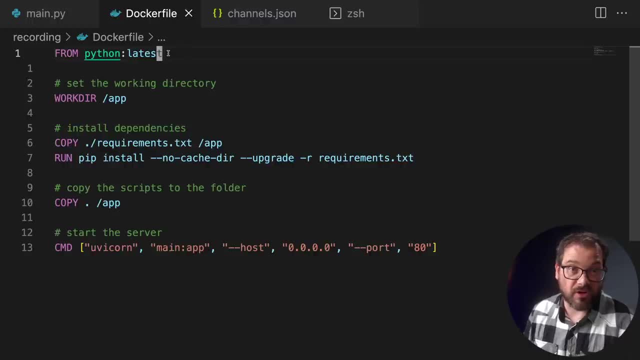 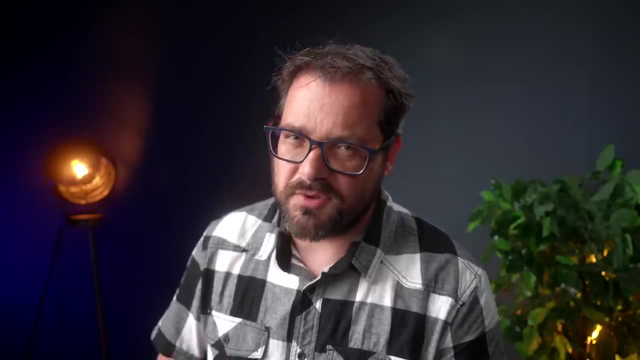 the latest version of the Python image. So this is a Docker image that has Python or already installed. It might not always be a good idea to just use the latest one, like I'm doing here. you might want to specify a specific version to make sure you're not getting any incompatibilities in the future. But for simplicity I'm just 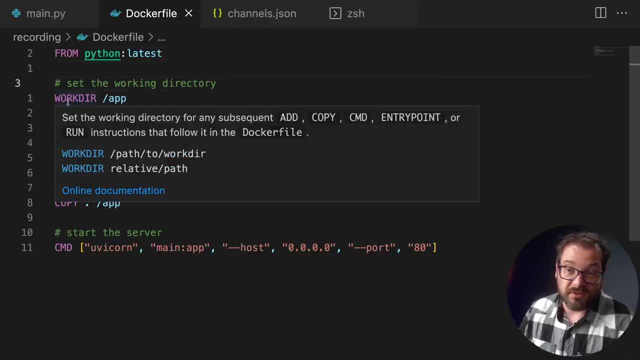 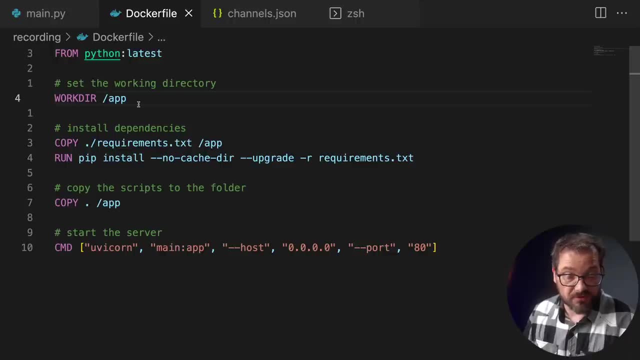 using the latest version of Python here. Then what I do is I set a working directory, So that's where all my files inside the container, so the container has its own file system. Within that I'm going to have a app folder where I'm going to put all the 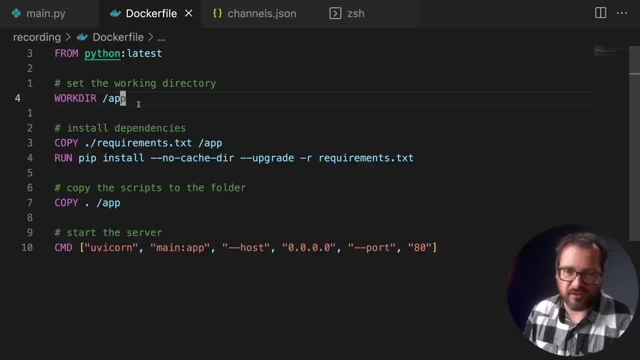 files that I need for my particular API. And that's done. That's the working directory. Then I install dependencies. So I'm copying requirementstxt, which contains the list of dependencies that I'm using in this project, to the app folder, which is my working directory, And then I run pip install. I'll come back to. 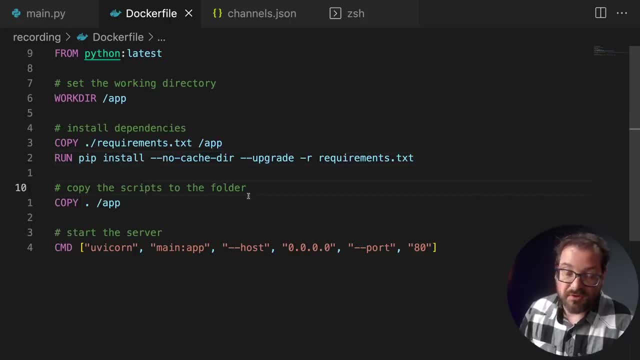 this again in a minute. After I've done that, I'm going to copy the script to the folder. So that means everything that's in the root folder, which contains mainpi and everything that I need. I'm going to copy it to the app folder And then, finally, I'm using. 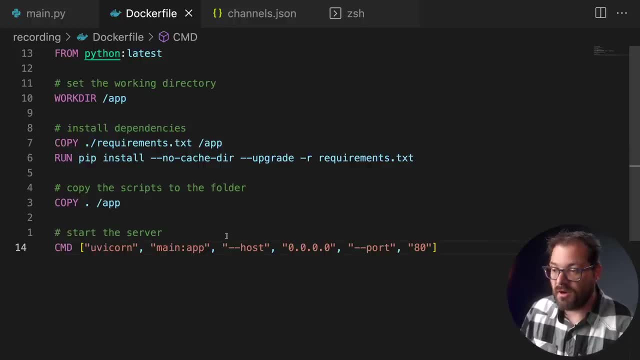 the command to start the server, which is uvicorn And internally in the Docker container. I'm running this on port 80, which is the default port to use for that. Also, you see, I don't have a reload option active here because there's no need to. Normally, if you deploy this. 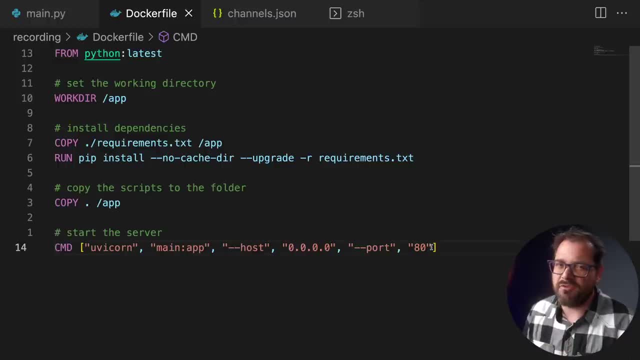 to the cloud. you won't change those files on the fly, But you will if you run this locally, And I'll show you how to do that in a different way in a few minutes. You might wonder why I'm copying requirementstxt separately here And then I'm going to copy this to the 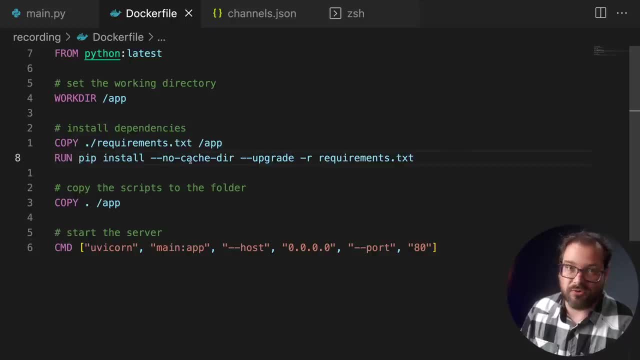 test and then run the install command. I could have also just copied everything, then run pip install and then start the server, right, That's the same thing. Well, that's true, But the problem is that Docker caches each of these steps. So if I would- 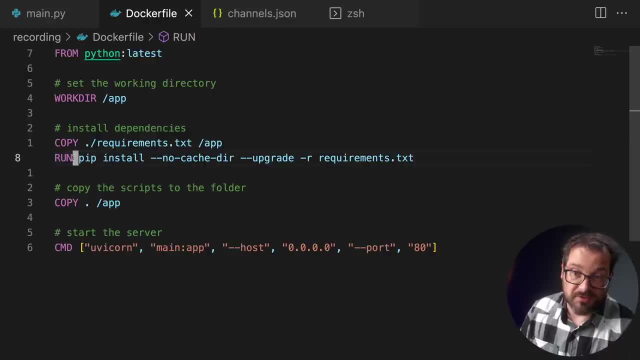 have copied requirementstxt here and then run pip install. that means that every time I make a change to the code, Docker is going to redo this step And that means it needs to reinstall the dependencies, which takes time. Dependencies don't change as often. I mean you might add a few. as you're developing your app, but they won't change as often as you change the code normally. so it makes sense to install those dependencies before you copy the rest of the code to the folder, so that when you change the code, docker has cached this dependency installation step and it simply copies the scripts. 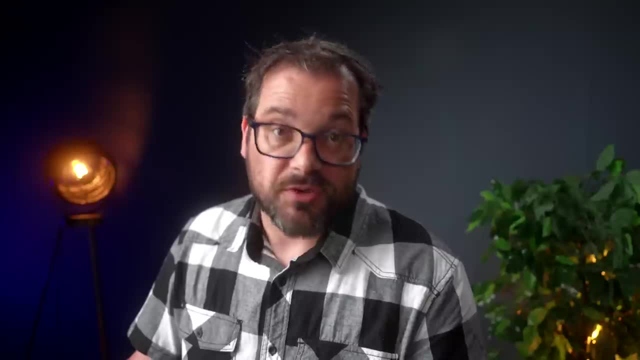 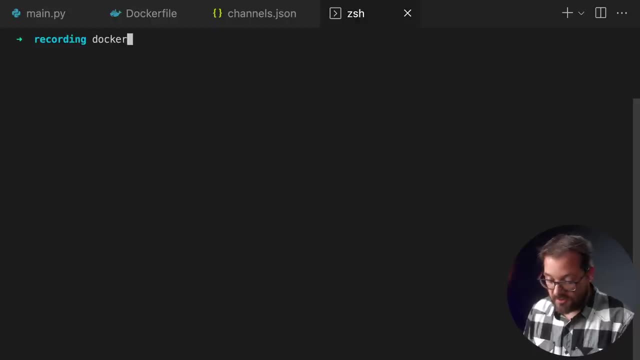 to the folder and starts the server, so that's just way faster. so once you have this docker file, you can instruct docker to start creating an image based on this file, and you do that using the docker command. so we're going to build it and i'm also going to supply a tag so that i can. 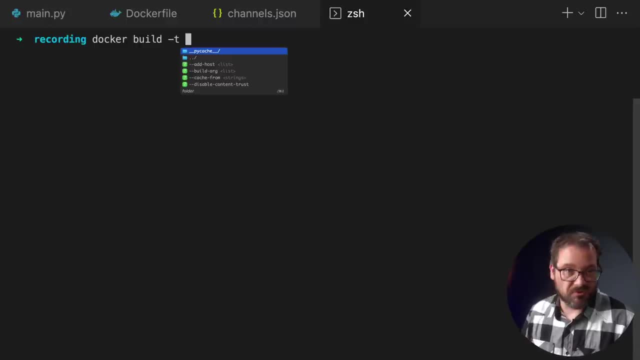 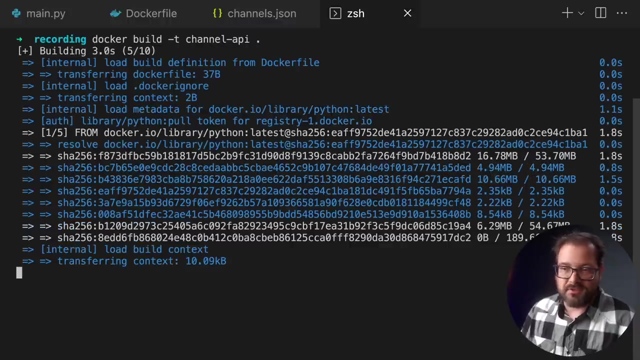 later on easily find this docker image back if i don't supply a tag. docker is going to invent some weird random name for me. i just want to call it- i don't know- channel api, and we want to build the image from the folder that we're currently in. so now you see, it's retrieving the python image. 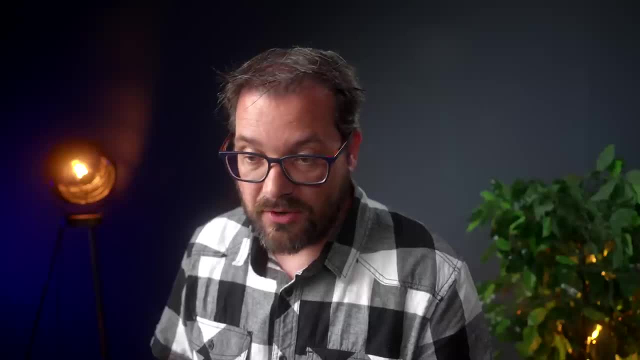 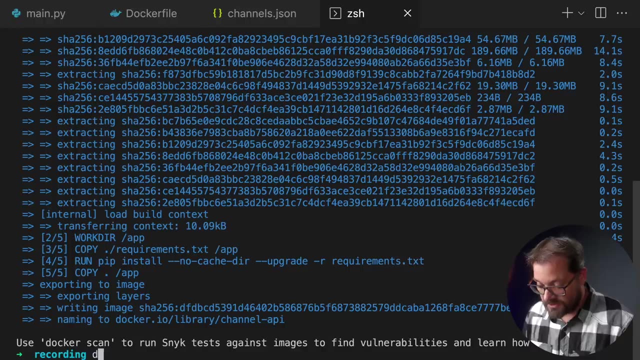 and it's going to build the docker image for me. so now that we have the docker image, we're going to build the docker image for me. i've built a docker image. i can create a local container to run the image locally on my machine. that's also using docker, but then with the run, and then i can pass a few options. so one thing. 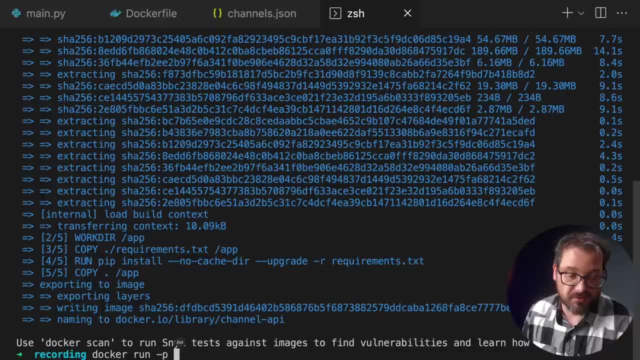 that i want to do is i want to specify the port that i'm going to publish this container on- so that's going to be 8080- just like i did when i was running the code locally, and i want the mapping from this port that i'm going to see in my machine to the port that's running internally. 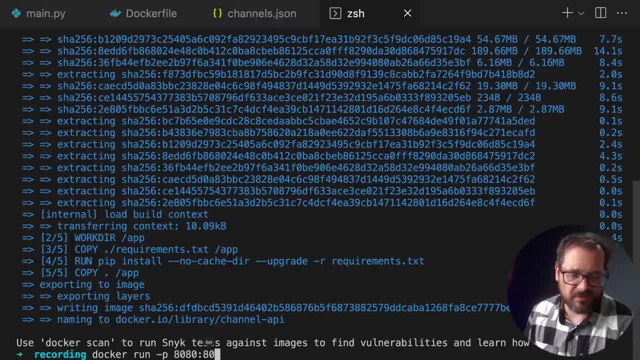 in the container, which is port 80, which is what we specified in a docker file, and i also supply the image, which is channel api. so this is what that looks like. there's one other thing i want to do, which is that i also want to run this detached, so that, after starting the docker container, i 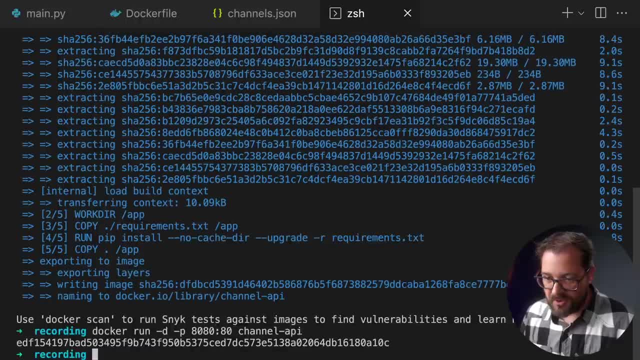 get my terminal back so i can write some commands here. so let's run this. and now we get also an id from docker. that's the container id, basically. so we can use this id later on to see if we can get our channel api back into the docker container. and we can run this. now we can see how the container 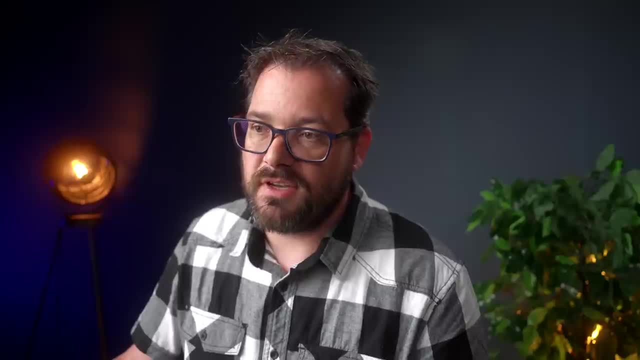 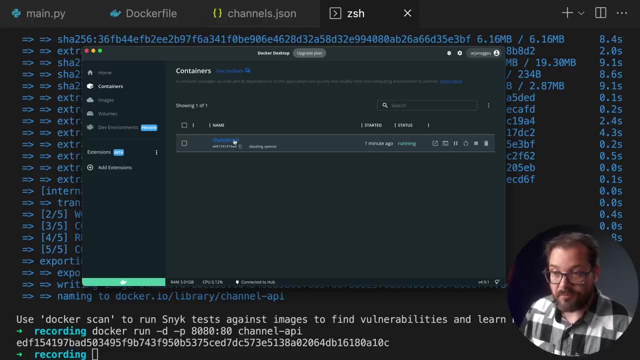 is running in the container, so we can see how our channel api is running, and you can also see this in your docker desktop application after you've installed that. so here you see, we have the channel api container that's going to be running. i can open this and then you can also see what's. 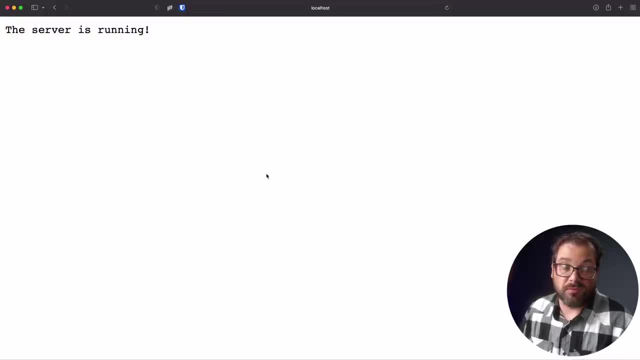 happening in the container right here. so let's go back to our server. so now i can perform the same request and the server is running. but now i'm accessing the data from the docker container and when I was running the code directly on my machine, I can access all the endpoints of this API. 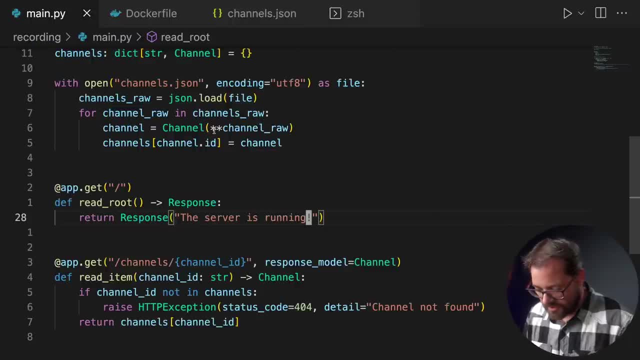 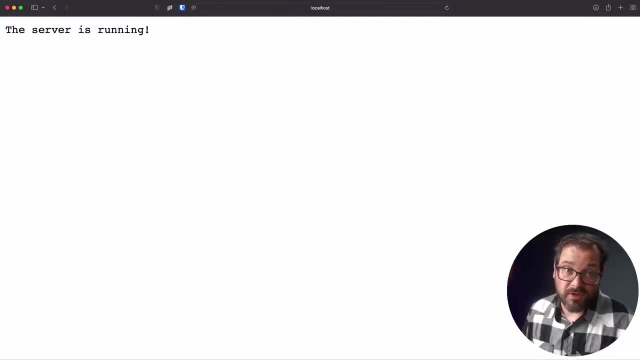 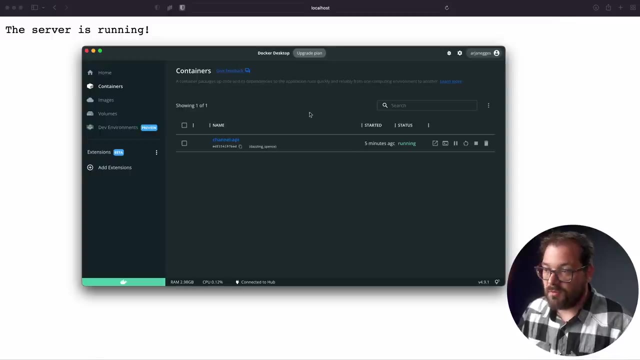 What happens if I change the code, For example, if I replace the exclamation mark here by a dot like so, then you see that my server is not automatically updated. So what I would need to do in my current setup is that I go to my dashboard. 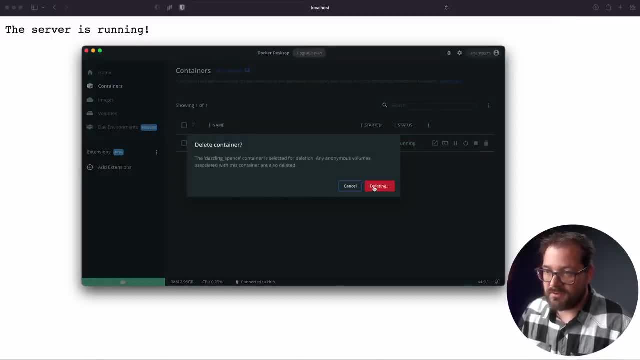 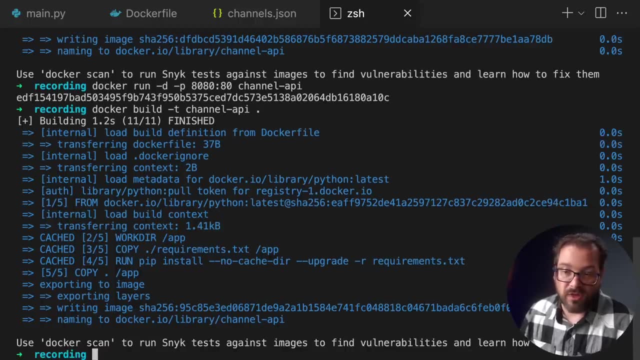 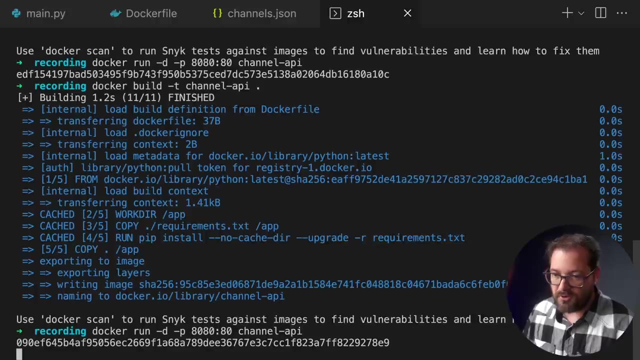 and I delete the container that's currently running and then I go back into my terminal. I'm going to build the channel API Docker image, which, well, it is going pretty fast because I cached the requirements, copying that you see here, And now we can run the Docker image again. 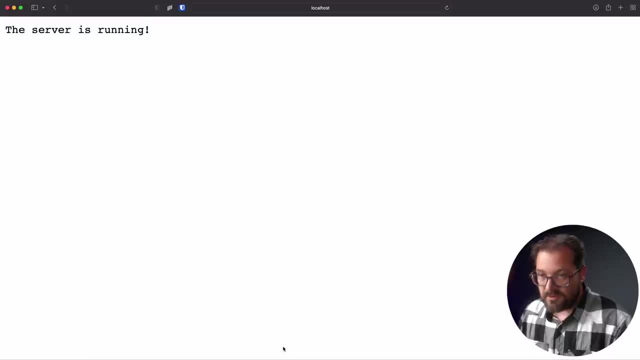 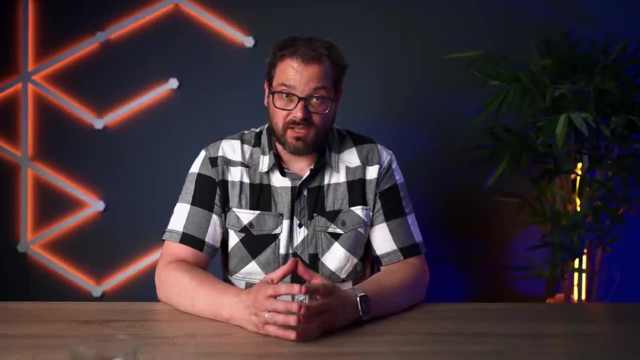 And if I now switch to my browser, then we get the new version of the code. This is not ideal, but fortunately there's a better option. When you deploy your code to the cloud, you'll need to build a server. You can build the Docker image just like I did before and tell Kubernetes. or whatever other container orchestration system you're using to update the running image to the next version. This is all part of your continuous deployment pipeline. If you're using GitHub, you can set this up with a GitHub workflow. If you're using Bitbucket, you can use a Bitbucket pipeline. And most alternatives will also have some kind of mechanism to start and run the deployment after committing and pushing a code change. The way I built and ran the container locally is not great. Every time I change something in the code I have to stop the server manually. rebuild the image and then restart the container. This is where Docker Compose comes in. It has two important features that make running your code locally in a Docker container really easy. You can supply a custom run command that restarts the server automatically when a file has been changed. 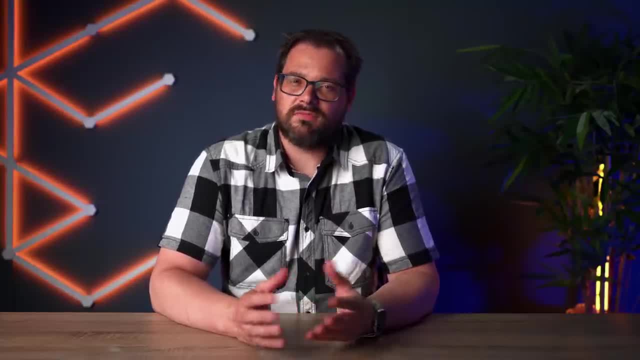 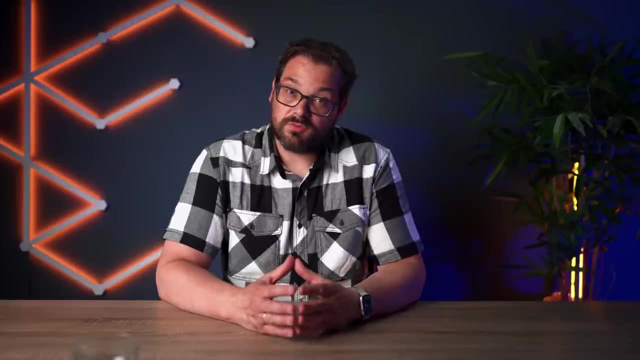 And you can sync a folder on your machine that's called a volume in Docker Compose terms to a folder inside the running container. You still need a Docker file- that I talked about before. but when you use Docker Compose you also need to supply a YAML file. 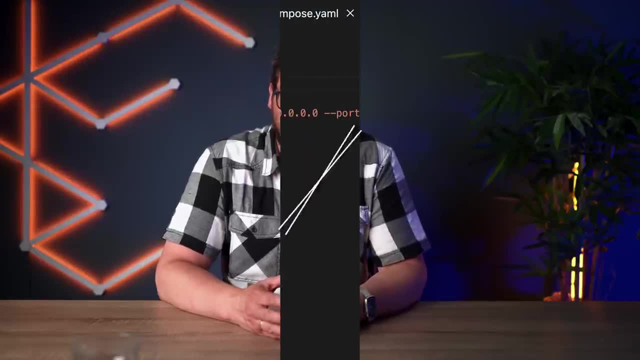 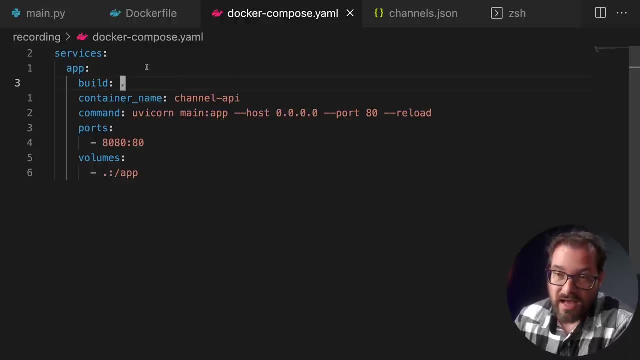 that contains the information that Docker Compose needs to run. Here you see an example of a Docker Compose YAML file. It's very simple. It contains a single app surface and that has a couple of properties. So the first one is the folder that we're using to build the Docker container. You don't necessarily need this, but if you want Docker Compose to build the image before you actually start the container which generally you want, it's useful to supply a build folder so you can actually do that. The second thing is the container name. 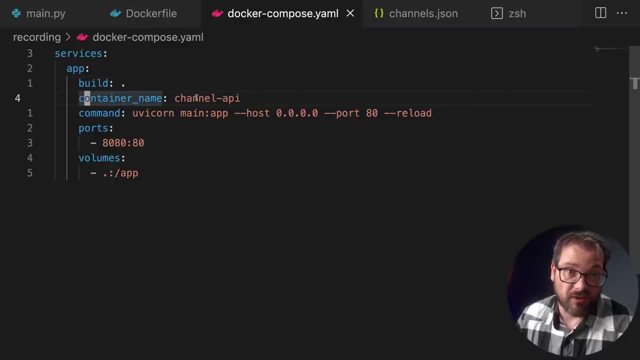 So that's when you create the container, we give it a name so we can easily find it in our Docker desktop. Then I'm supplying a custom command here which is uvcorn, etc. etc. port 80, so that's all the same. 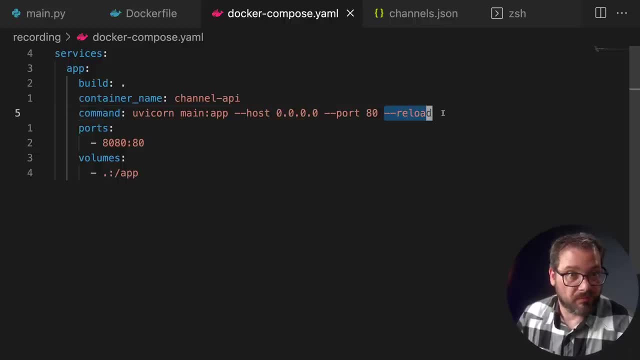 but I am supplying the reload option here because we want to reload, restart the server when our code has been changed, And what this does is this: replaces in the Docker file this command that we have here. So Docker Compose still uses the Docker file. 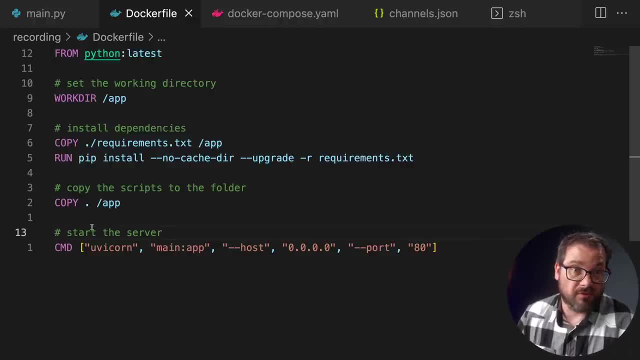 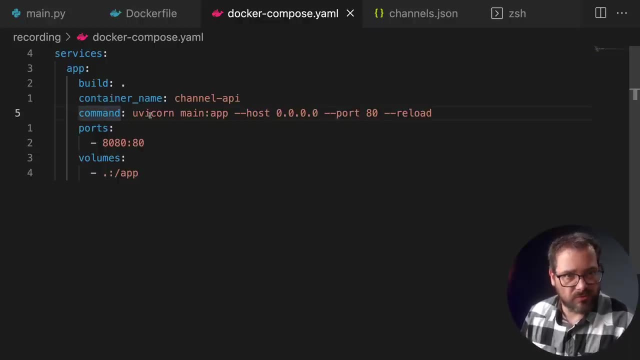 but it replaces some of these commands with some of its own custom things. So in this case we're replacing the command because we want in Docker Compose, which is, we'll only use this locally- we want to make sure that if the code changes, we restart the server. 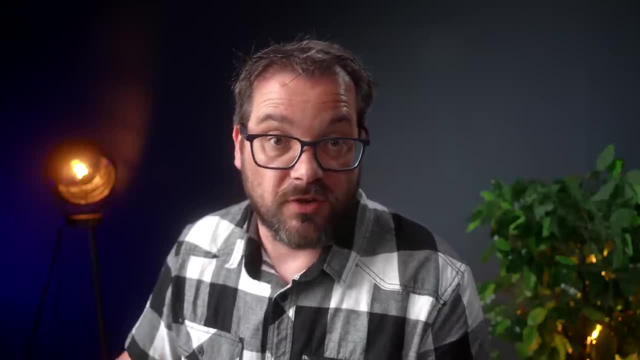 When we deploy this to the cloud. this is not important, because the code doesn't change. There will be a new deploy in that case- but locally we want this to happen, so that's why we override the command. We also do the port mapping. 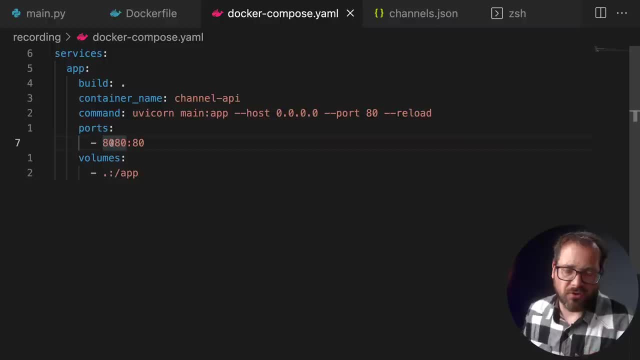 So we're saying that we, to the outside, outside of the Docker container, we want to expose port 8080, which is what we have at the moment- and internally that maps to the 80 port which is used in the Docker container. 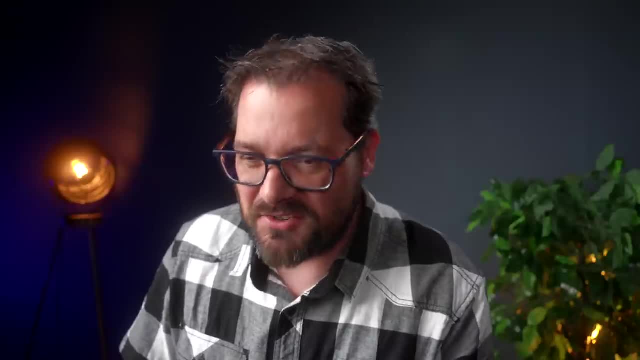 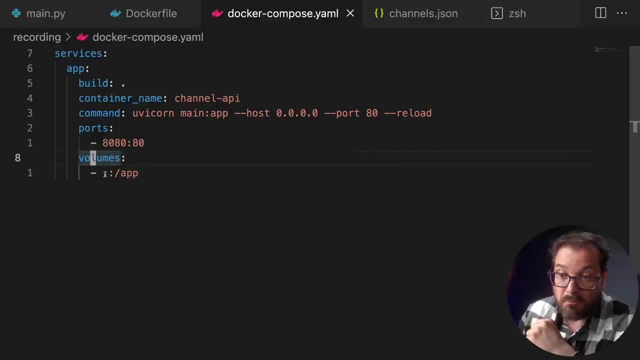 and that's also supplied here as part of the command. And this is the bit of magic that makes everything come together really nicely is that we're defining a volume, And what I'm doing here is I'm defining a mapping between the current folder and the slash app folder inside the Docker container. 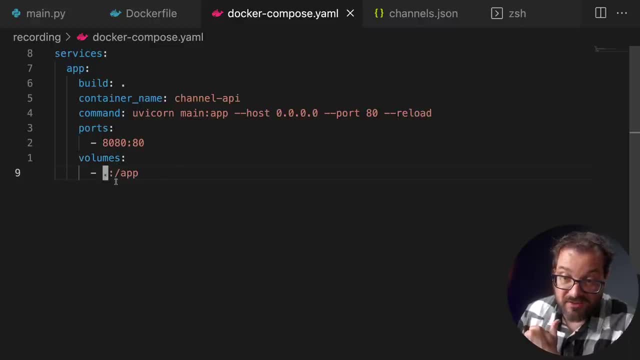 And what this does is really neat. This means that if we change anything in this folder, in our project folder, then it's going to sync those changes automatically to the app folder And because it syncs those changes, the files are going to be updated. 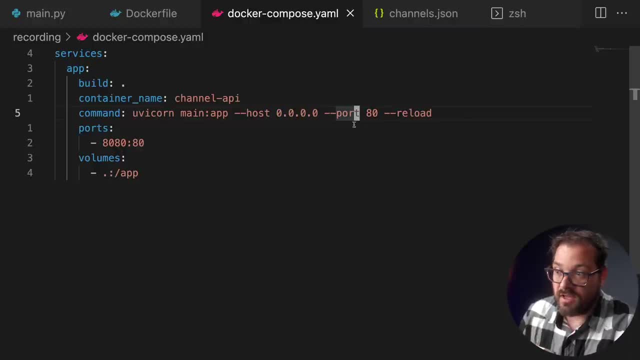 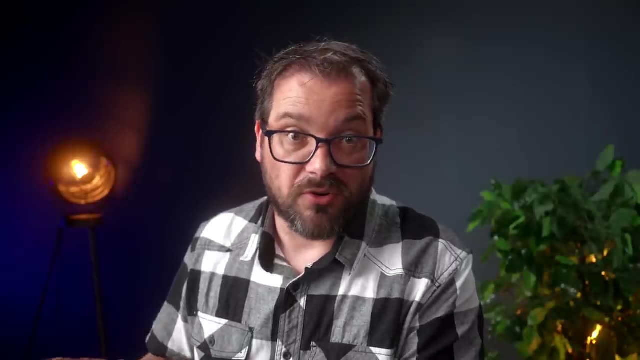 Our UV Gordon commands will detect that change and it's going to restart the server because of this command. So when you put all this together, you now have a system where you're able to run your API in a Docker container, but you can change the code and when you do, save the file. 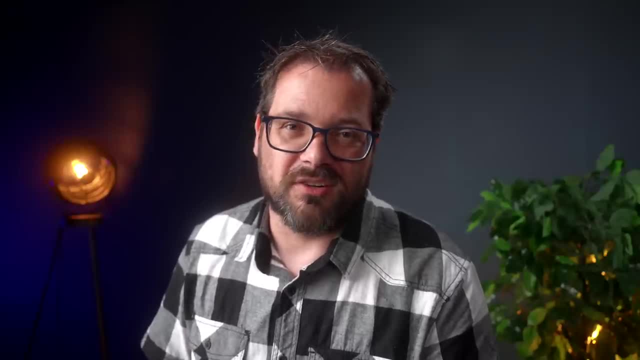 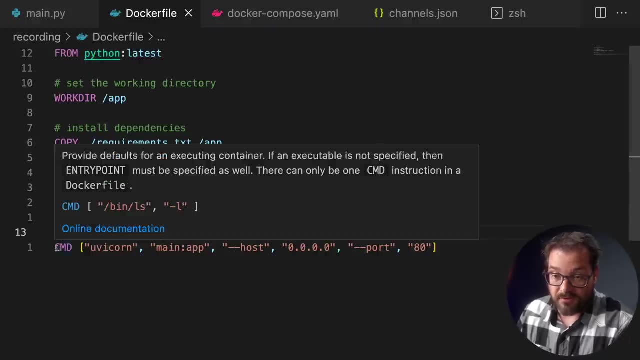 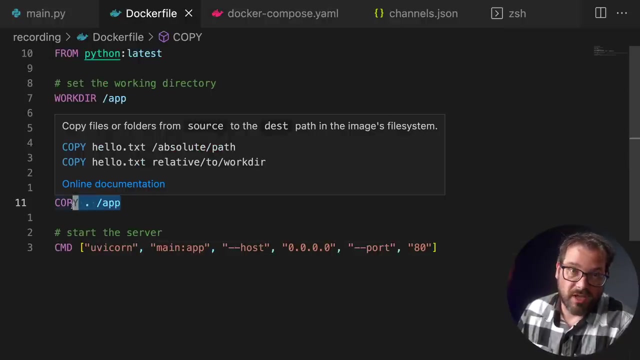 it's going to automatically restart the Docker container for you because of the volume syncing option that I've added here. So a custom command that overrides this command right here and the volume that actually overrides the copy behavior that we have here. So let's try this. 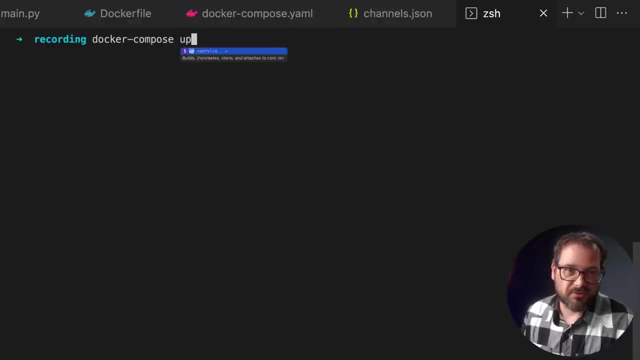 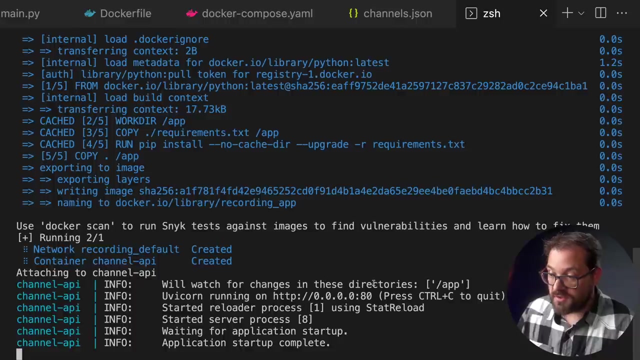 So we have Docker compose And we're just instructing it to update automatically. So this does the syncing and automatic restarting of the server, And we also want to build the container for the first time. So now you see that it's going to watch for changes in the directory slash app. 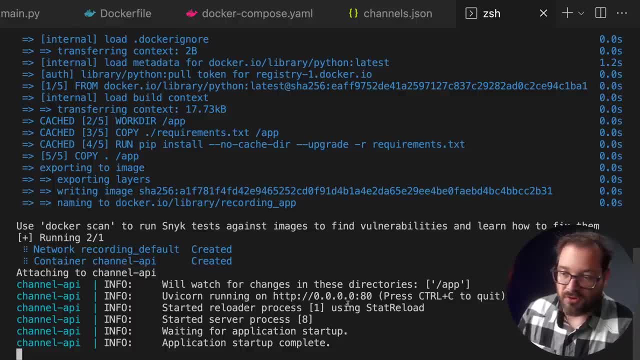 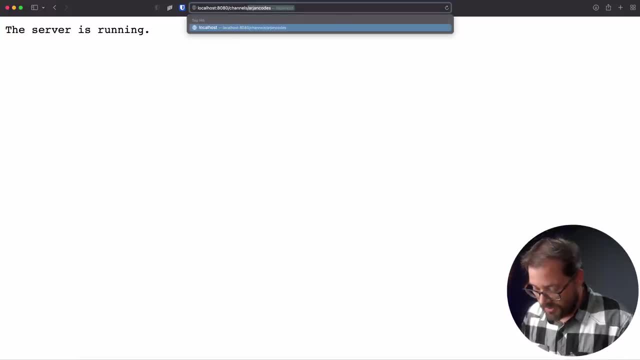 and UV Gordon is running locally inside Docker on this port. So now when I go to the browser I can show that the server is running. Let's also get some channels information again like so, And that also works. So that's nice. 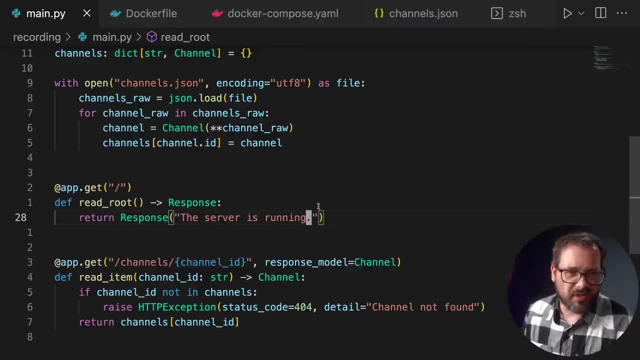 And now when I go to my main file, let's say I replace the dot again by an exclamation mark like so: So I'm changing the code in the server, And then we see here that UV Gordon detected a change here, and then it's reloading. 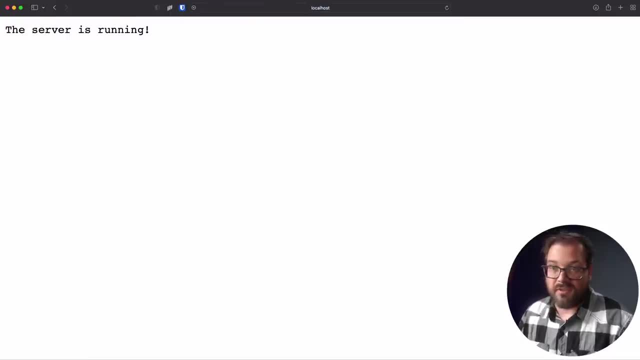 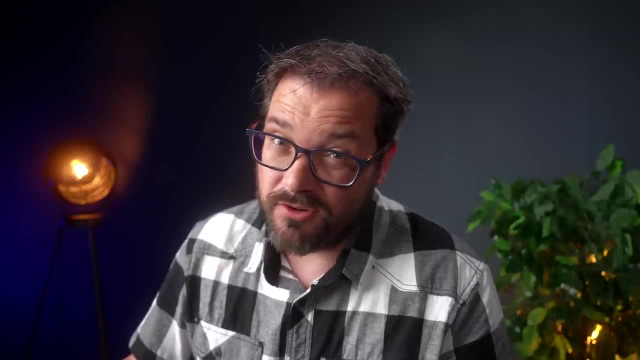 So now, when I go back to my browser again, you see that we get the results that we expect. So now it's an exclamation mark again. A final thing that I want to show you is how to deal with changes in data, because currently, 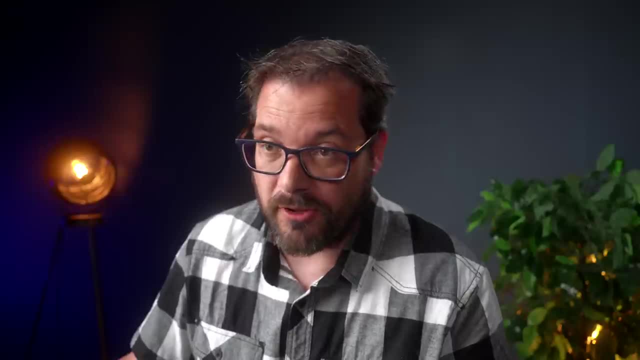 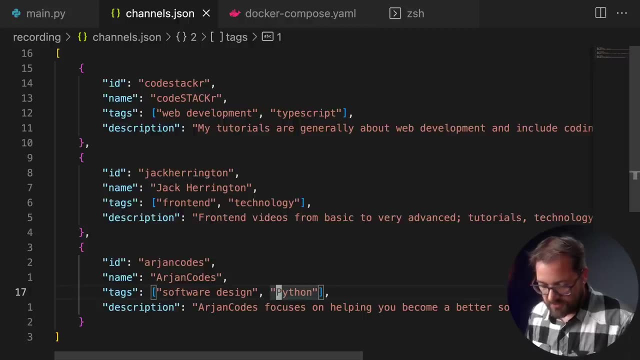 UV Gordon only restarts the server when I change the Python file. For example, if I go into my channelsjson file and I change Python to use a capital letter- P, like so- and then I go into my server and I request my channel information. 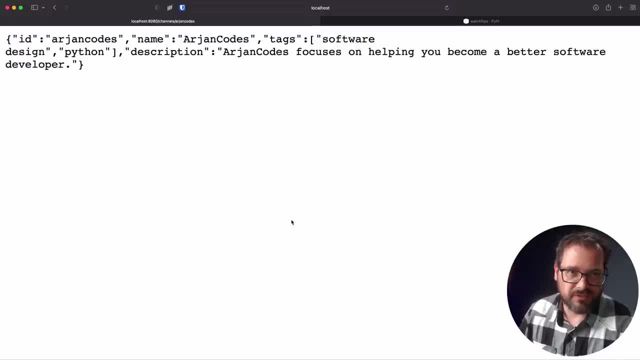 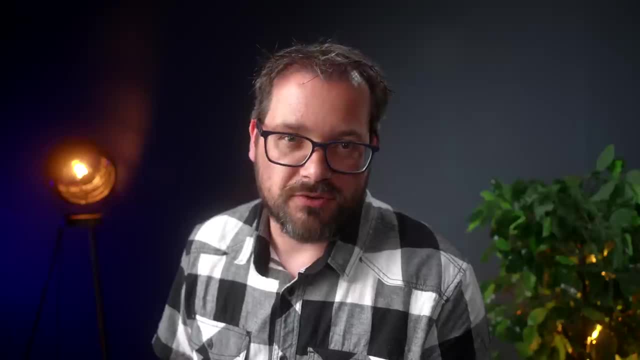 nothing has changed, because UV Gordon only detects changes in pi files. So how do you fix this? Let's stop this server that's currently running, and what you need to do is to specify more precisely to UV Gordon the kinds of files that it needs to fix.